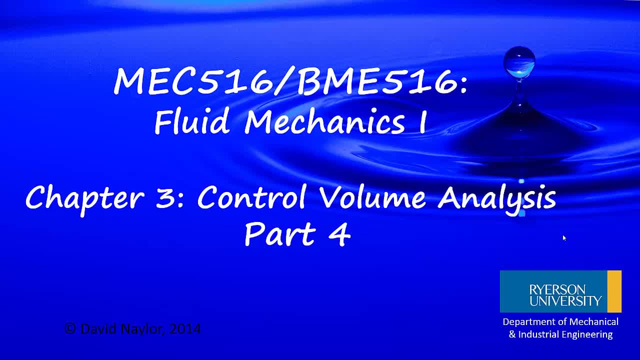 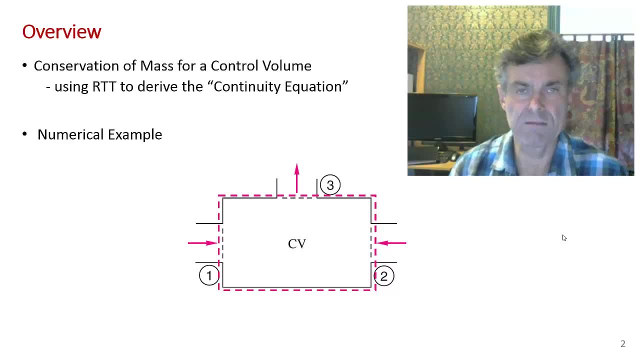 Hi, this is chapter 3, control volume analysis, part 4.. In the previous video, we talked at great length about Reynolds transport theorem, which allows us to convert a system analysis to a control volume analysis, And what we're going to do now is use Reynolds transport. 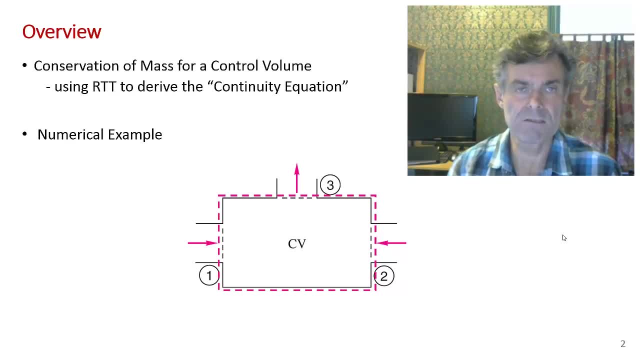 theorem to derive the conservation of mass equation for a control volume. And I should point out that in fluid mechanics the conservation of mass equation is usually referred to as the continuity equation. So conservation of mass and continuity equation mean the same thing. And then we're going to do a very simple numerical example. 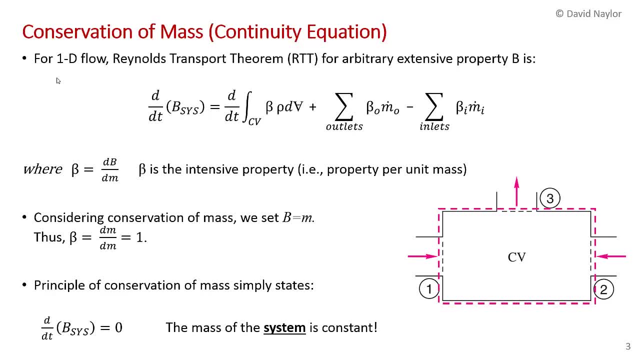 In the previous video we spent a substantial amount of time deriving Reynolds transport theorem, really with a focus on one-dimensional flows, And so I've rewritten here the Reynolds transport theorem for a one-dimensional flow, for this arbitrary extensive property B- And remember, an extensive property is just a property that depends upon the mass. 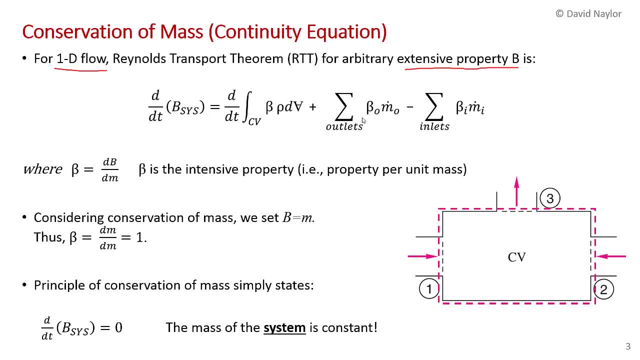 or extent of the system. So what we have here is that the rate of change of B within the system- so this is the fixed amount of mass that's passing through the control volume- equals the rate of change of this quantity. So the rate of change of B within the control volume plus the rate at which B flows out. 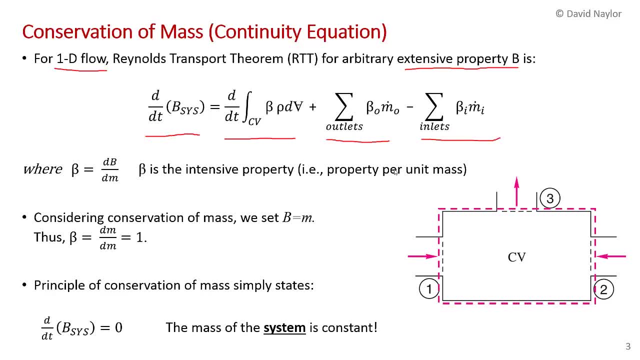 minus the rate at which B flows in. And remember this property, beta. here is the intensive property, the corresponding intensive property, and it's defined as db dm. So for example, if B has momentum mv, then the intensive property would be v. 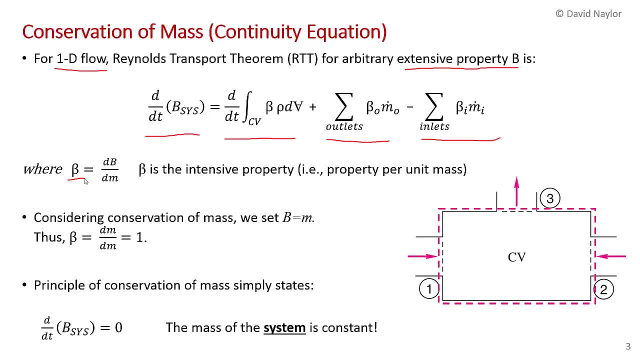 In this case we're considering conservation of mass, so we're thinking about mass flowing in and out of the control volume. So in this case we're going to use, we're going to set B equal to m. So now we take the derivative db, dm, we just get the beta equals one. 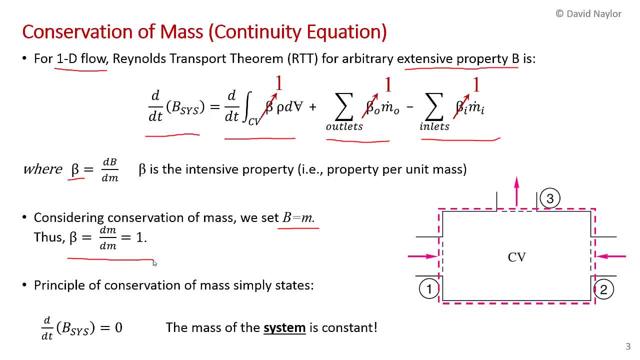 And so we can set beta equals to one in each of those terms. Now, the general principle of conservation of mass says that— the mass of a system- and by definition a system is a fixed quantity of mass. it can't change mass, can neither be destroyed. 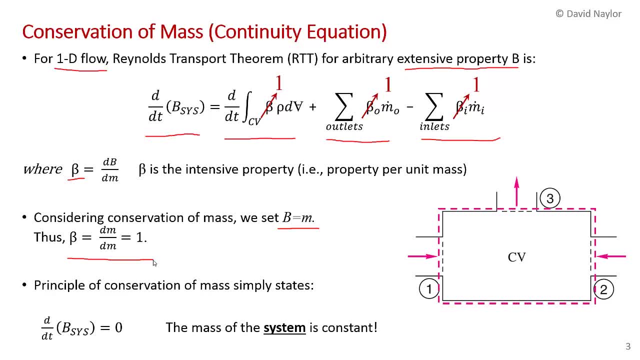 nor created neglecting relativistic effects, and so for general engineering purposes the mass of the system is constant, so we get that the rate of change of the mass of the system with time has to be zero, so we can set that the term on the left hand side to zero. 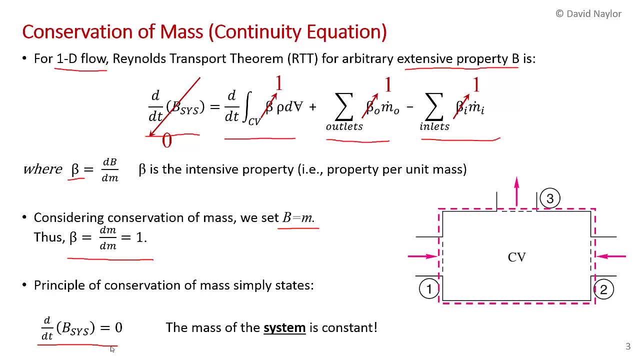 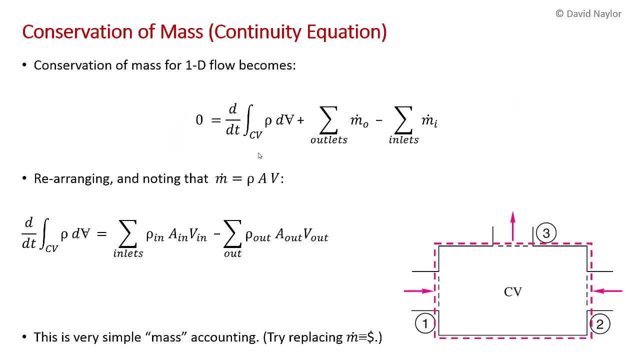 now, in the next slide, what we do is we rewrite this with that beta set equal to one and the left hand side set equal to zero. so here's the resulting equation for conservation of mass for a one-dimensional flow: we have the left side equal to zero. 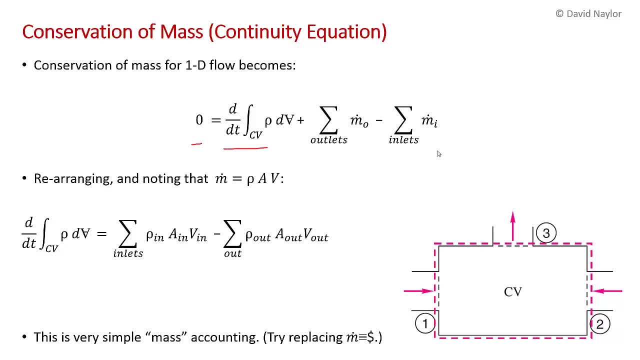 we have the storage term and then we've set beta equal to one, so we just have the mass flow out minus the mass flow in, and we noted in a previous video that the mass flow rate is just the density times the cross-sectional area, times the average velocity in a duct or a pipe, and so 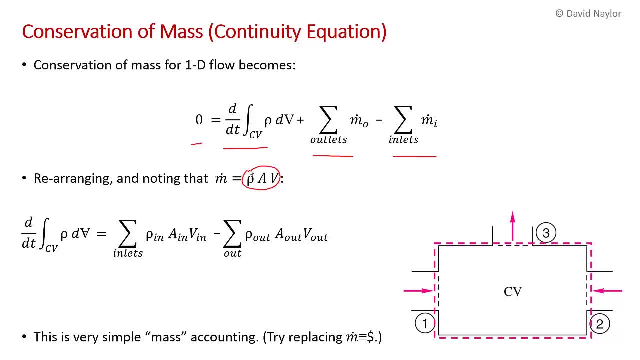 I've made the substitution here. I've made the substitution for rho, av, for the mass flow rates, and what we have down below then is on the left side we have the rate of accumulation. I've done a little rearranging. the rate of accumulation of mass within the control volume equals the rate of. 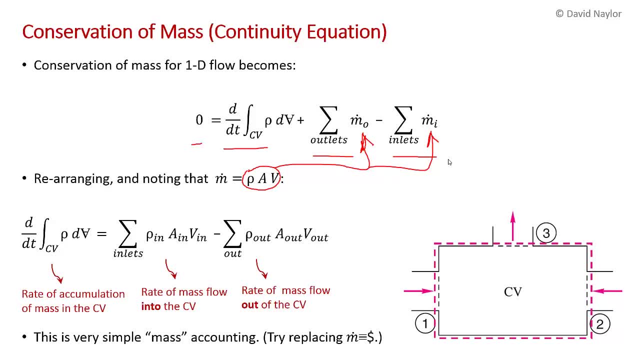 mass flow into the control volume minus the rate of mass flow out of the control volume. now, if you've done in thermodynamics, you probably already have seen this equation, but, as I pointed out the other day, the biomedical students don't get thermodynamics. Now I should point out that we could have come to this without. 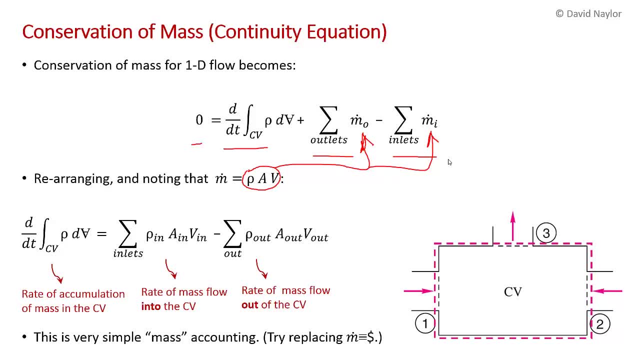 using Reynolds Transport Theorem. it's really very simple, mass accounting in this case, and one way to sort of remember it is to just think about replacing the mass flow rate with money. you know, if you think about your bank account, it's just simple, it's just like the accounting. 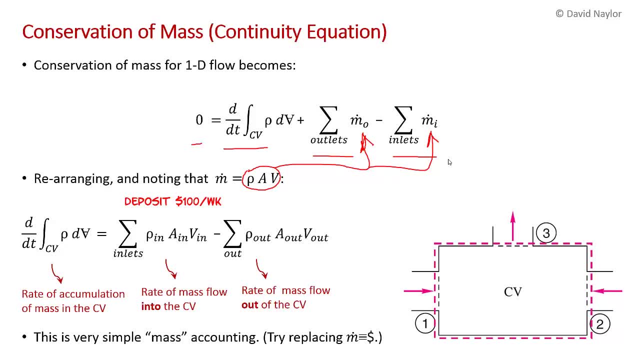 in your bank account. you know, if you deposit 100 dollars a week week and you take out $25 a week- and you do that- we couldn't weekend week out- your bank balance is going to go up at a steady rate of $75 a week. so you can see. 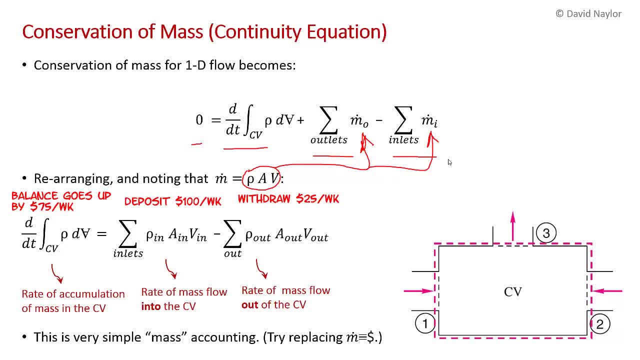 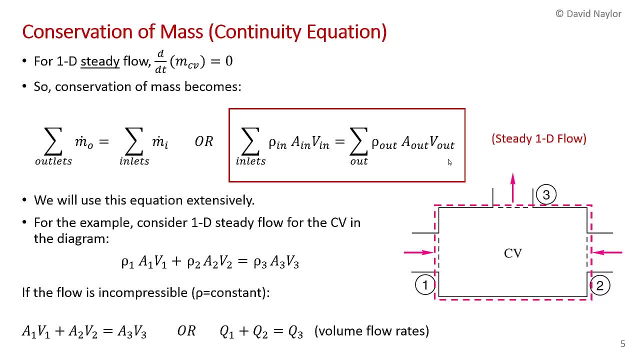 it's a very intuitive, simple concept: continuity. now, if the one dimensional flow is steady and steady flows, that means that you know nothing is changing in time. so time derivatives go to zero, and so the rate of the rate of change of the mass within the control volume. there's going to be no storage of its. 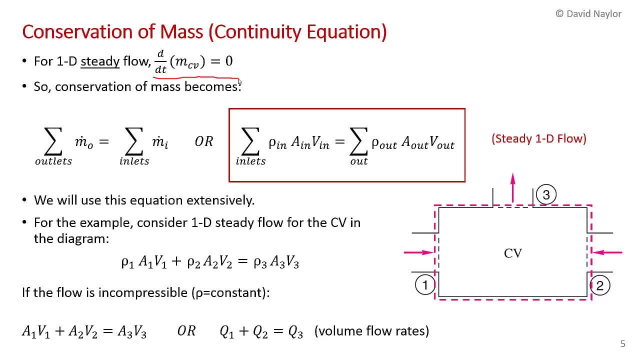 steady, the rate of change of the mass within the control volume equals zero. in that case you can set the storage term to zero and you just get that the rate of mass flow out equals the rate of mass flow in. and of course you could have any number of inlets and outlets from your control. 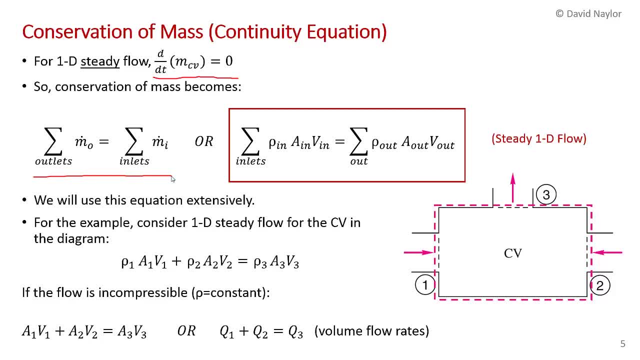 volume. so you've got a sum over the inlets and the outlets, and so that's for steady, one-dimensional flow. so row in a in V in has got equal, summed over all the inlets has got equal. row out a out V out, summed over all the outlets, and we're. 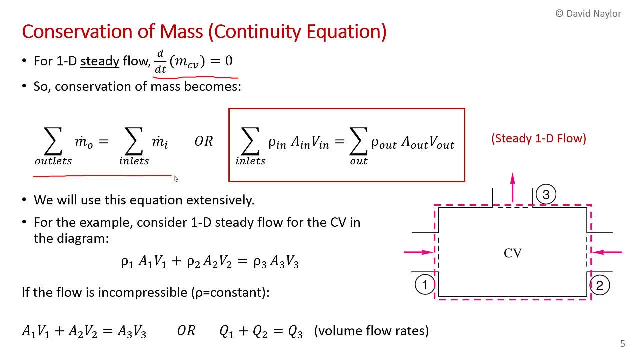 going to extend, use this equation extensively in the rest of the course, and so, for example, for this control volume that I've shown over on the right-hand side, we've got inlets at one and two and an outlet here three. so in that case you just say this: 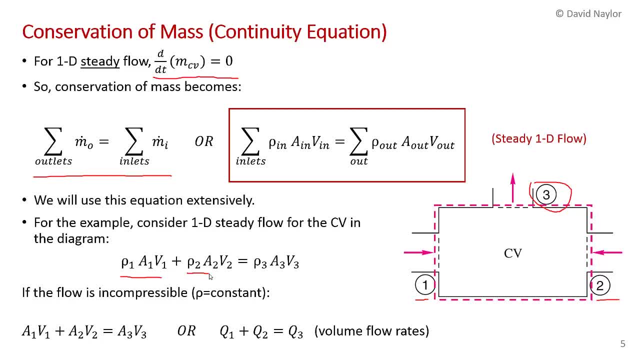 is the mass. this is the mass flow rate at one plus the mass flow rate at two, has got equal the mass flow rate at three if the flow is incompressible. so that would be the general form that you use for a gas. but if it was a, if it was a liquid? 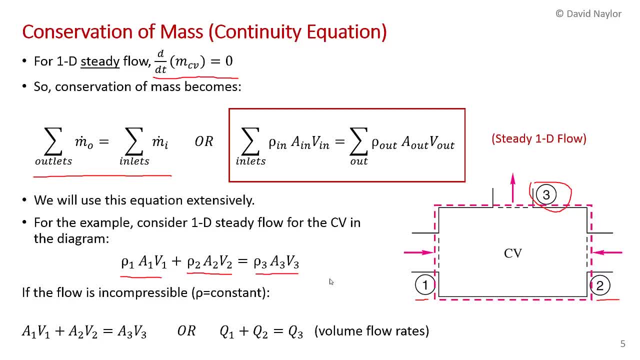 and the density is a constant, doesn't depend on pressure, then if that's the case, then you can. you can cancel the densities here, but only only if it's a in compressible fluid, only if it's a liquid, and in that case you just end up with that volume. flow rates are. 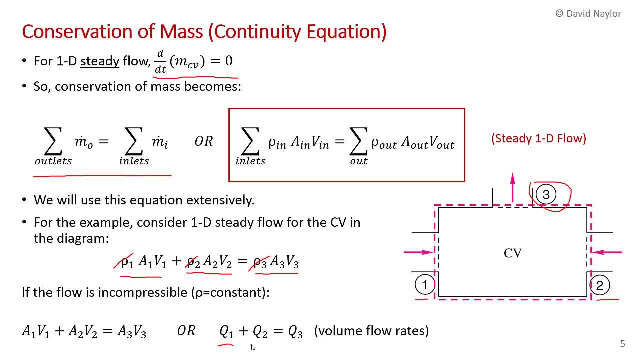 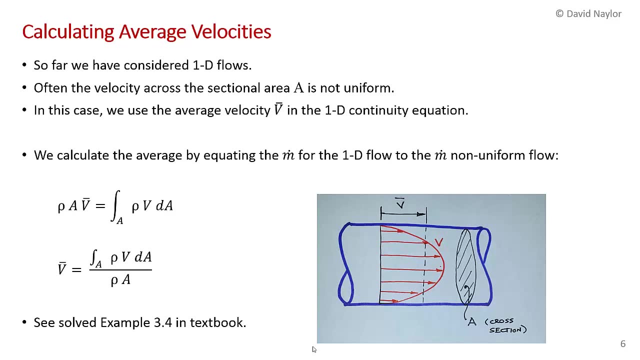 conserved. so the volume flow rate at one plus the volume flow rate at two must add up to the volume flow rate at three. so that's very simple, but that's only for in in compressible fluids. now, so far i've been considering sort of ideal. 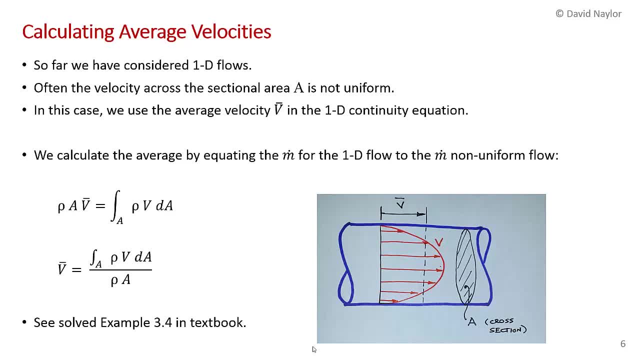 one-dimensional flows. but I say here often the velocity across the cross-sectional area is not uniform, but in reality it's. it's never uniform because you have the no-slip condition at the boundary, so the velocity at the surface of the pipe or duct is always. 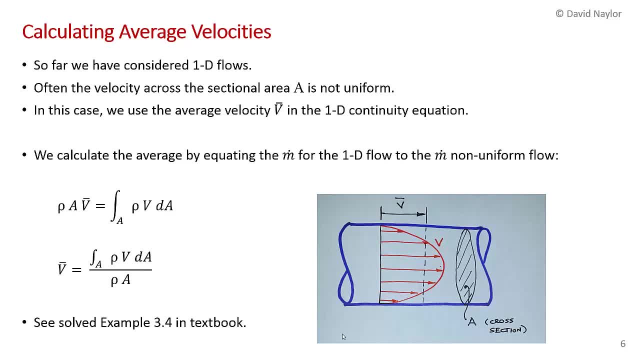 going to be zero and I've drawn a pipe here- sketch the pipe down here- where we have laminar flow and we have a parabolic velocity profile, and in this case, if you want to apply this flow to one-dimensional equations, we have to put in the average velocity here, and so we calculate the average velocity by. 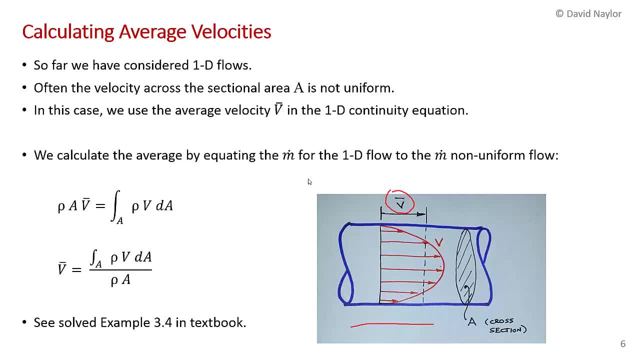 integrating the mass flow rate and setting the mass flow rates, or the one-dimensional flow, equal to the mass flow rate for the none, non-uniform flow. so looking at this equation over on the left-hand side, rho a V bar. that's going to be the mass flow rate. 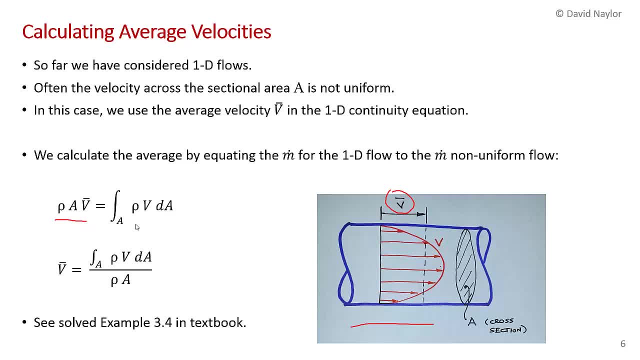 for the one-dimensional approximation, that's got to be equal to the integral of Rho V da, which is the local integrate, the local mass flow rate across the area, the cross-sectional area of the pipe. and so then, rearranging, you just get the V bar equals the integral of Rho V da integrated across the pipe, divided by: 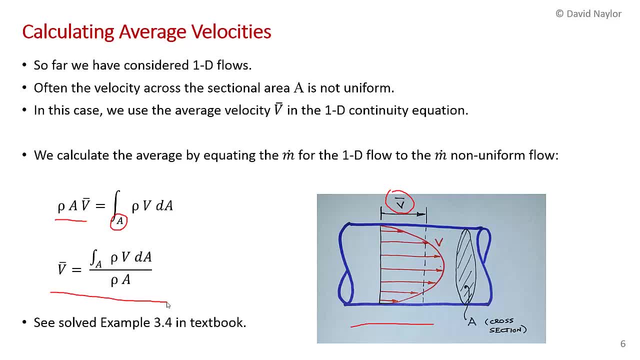 Rho and then a is the total cross-sectional area of the pipe. if the pipe is round, you've seen in previous examples we use a little annular area for da, which is 2 pi R, dr. there's a nice solved example in your textbook. check out example 3.4 in the chapter 3 where they solve the average. 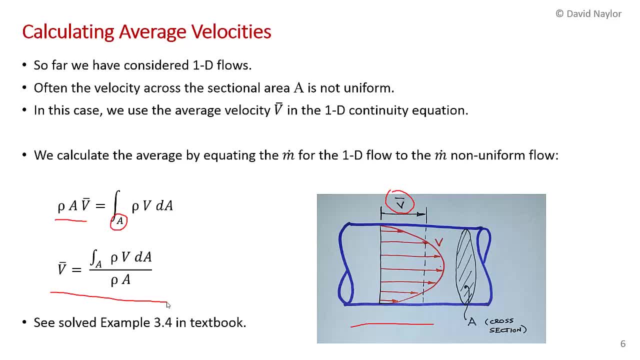 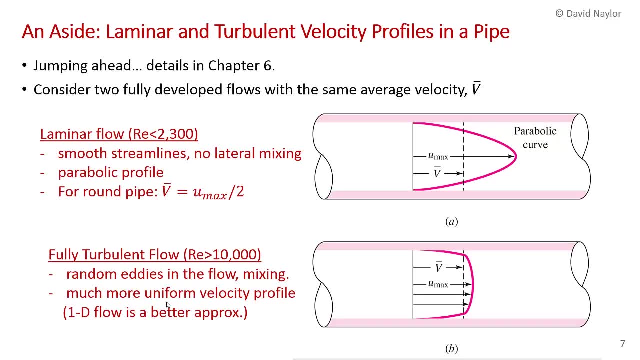 velocity. it's fairly straightforward, I think. as an aside, I thought I'd see a few more examples of the Rho V da and then I'll show you some examples of the different velocity profiles you get in laminar and turbulent flows and pipes. this is really jumping ahead, but it's worth mentioning it now, and then you'll. 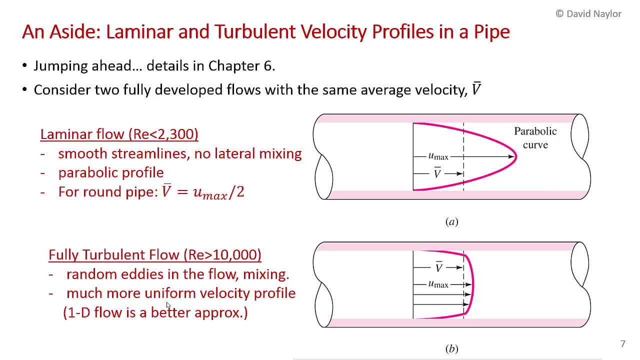 hear it again when we when we talk about the details of pipe flow in chapter 6. so if you consider two fully developed flows- and by fully developed I mean these are flows in a pipe that are well away from the entrance of the pipe, so the velocity profiles become fully established in the pipe. if you consider 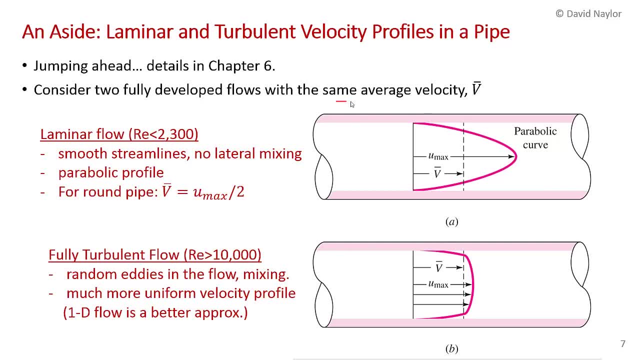 two fully developed flows with the same average velocity, V bar. if you have a low Reynolds number then you get laminar flow and I mentioned that in a previous video. I think there's one of the introductory videos from chapter 1. it turns out that for pipe, if your Reynolds number is less than about twenty three, 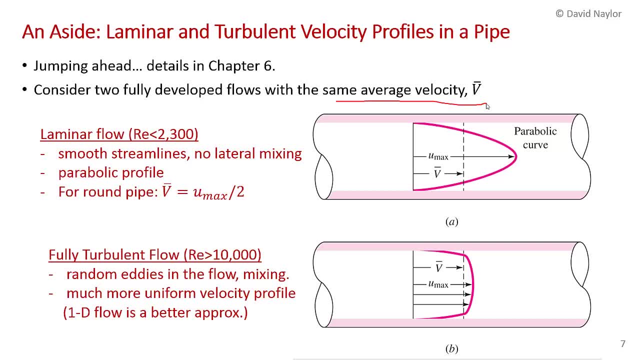 hundred, and that comes from the famous Reynolds experiment that you're going to reproduce in the lab in one of the experiments. if there, if that Reynolds number is less than twenty three hundred, you get really smooth flow, no eddies, no lateral mixing across the pipe and you end up with a velocity profile. 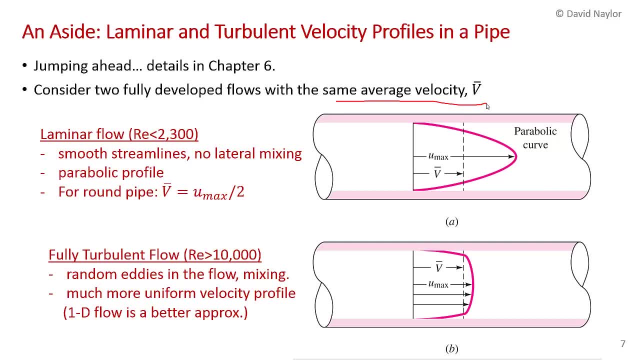 across the radius of the pipe. that's a parabola. and indeed later on in the course, I think in the next chapter, we're going to derive the equation for laminar flow in a pipe, and in that case I'll tell you the result. what you get is that: 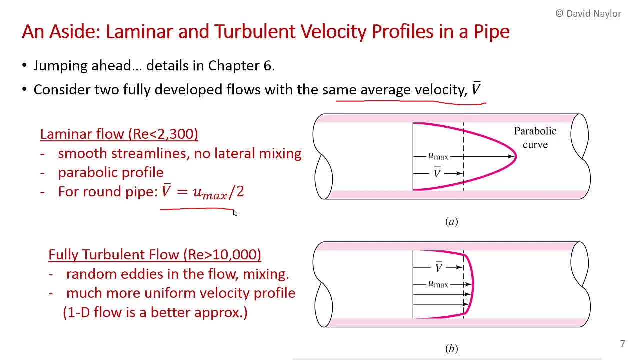 that that the maximum velocity here is this. this maximum here is two times, two times the, the average value. that's for laminar flow, where you get a parabolic velocity profile, but when you increase the Reynolds number and you get into a really fully turbulent flow. so we have 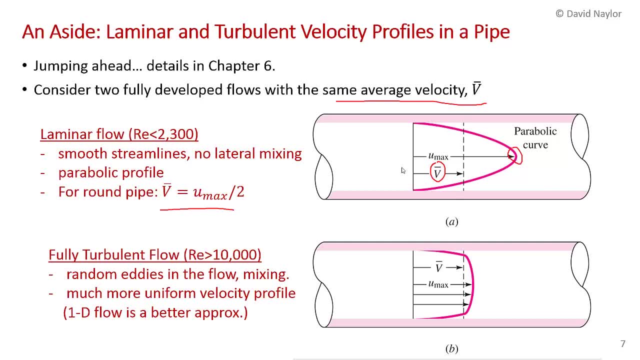 strong mixing that corresponds to a Reynolds number around ten thousand or greater. then you get a lot of eddies in the pipe, random mixing, lots of mixing from the center of the pipe towards the wall and that transport, extra transport of momentum by the mixing, produces a much 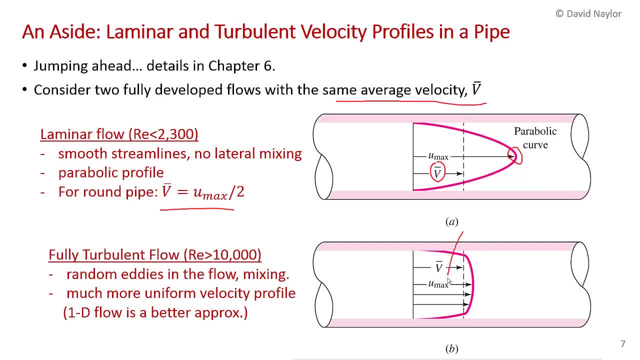 more uniform velocity profile and yes, you can see here we don't have the that huge difference anymore between the average and the maximum velocity of the pipe. so turbulent flow in a pipe is actually a better approximation of a one dimensional flow. much more uniform distribution. that's probably more. 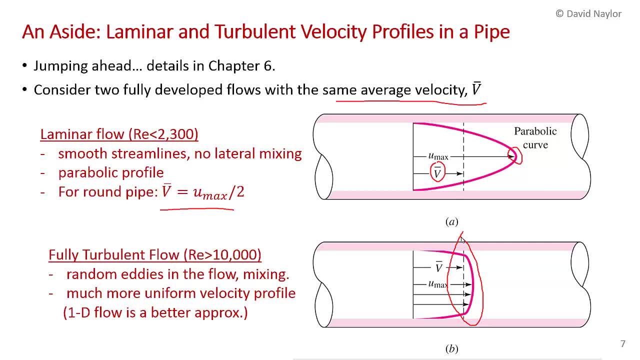 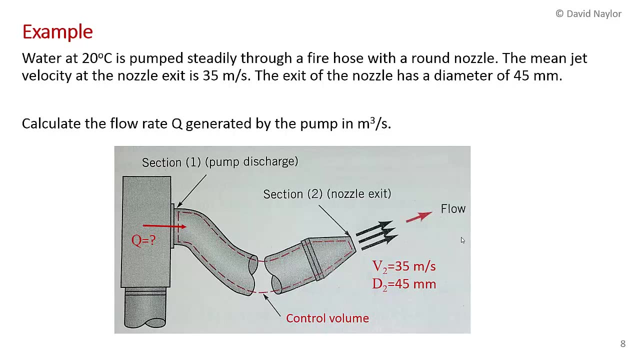 information than you need right now, but it's worth mentioning it, since we were talking about average velocities and we'll come back to this issue when we talk about chapter six. I'd like to end the video with a short, simple example. What I'm considering here is water. 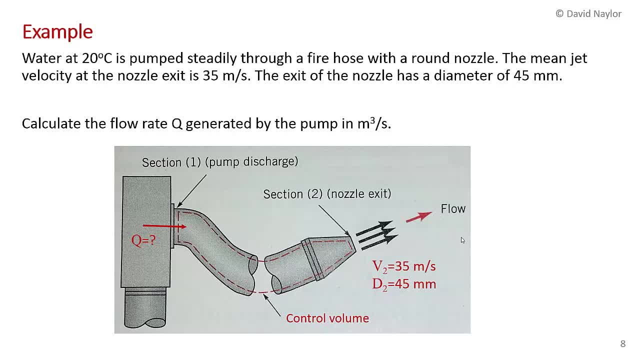 that's being pumped steadily through a long fire hose with a nozzle at the end and the mean jet velocity at the nozzle exit is 35 meters per second. and I've written sort of the conditions here: 35 meters per second and the exit of the nozzle this diameter here, that diameter there. 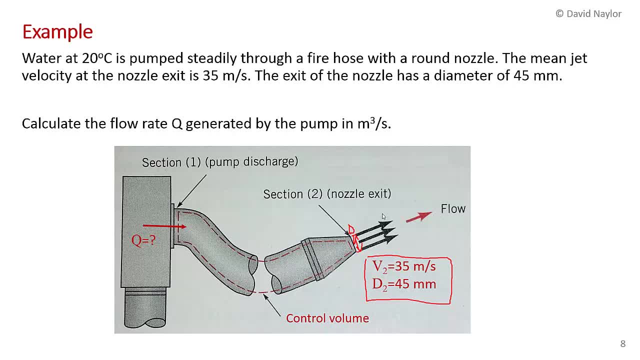 is 45 millimeters and what we want to calculate is the volume flow rate that has to be generated by the pump in cubic meters per second. so we're after the, the volume flow rate here that's being generated by the pump. I've drawn a control volume, the dashed red line. 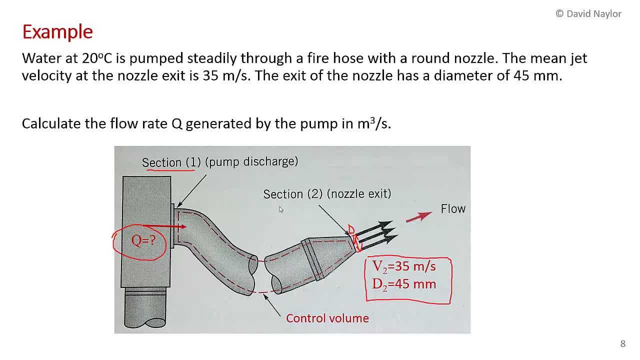 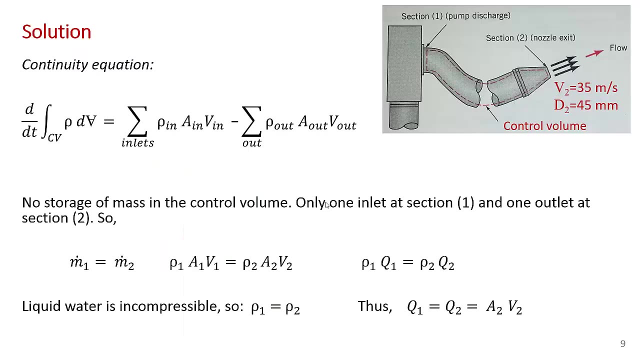 and we're going to consider the inlet to be section one and the nozzle outlet is section two, and we're going to, you know, use one-dimensional approximations using the average velocities at those sections. This is a very simple but important example. so I've written the continuity equation. 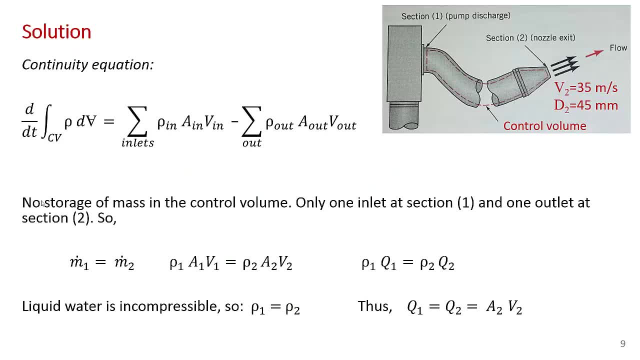 here we have the, the rate, the rate of storage of mass within the control volume equals the rate at which mass flows in and we're told it's a steady flow. so if it's steady flow, time derivatives here go to zero, so we can get rid of that term. we just have, as we discussed previously, that the 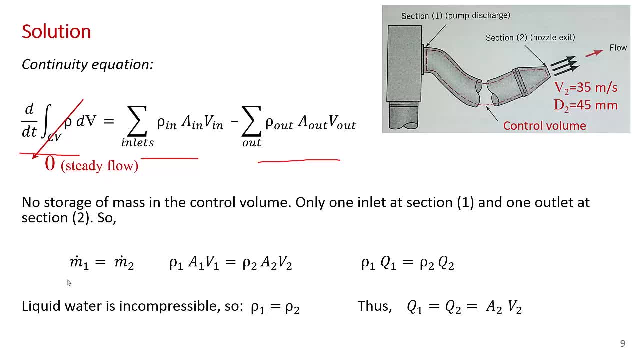 mass flow rate at section one equals the mass flow rate at section two. so rho one a one v one, the average velocity at section one, equals rho two. a two v two, the average velocity of section two. We can combine these two terms. remember av is just the volume flow rate, so we can rewrite them at: 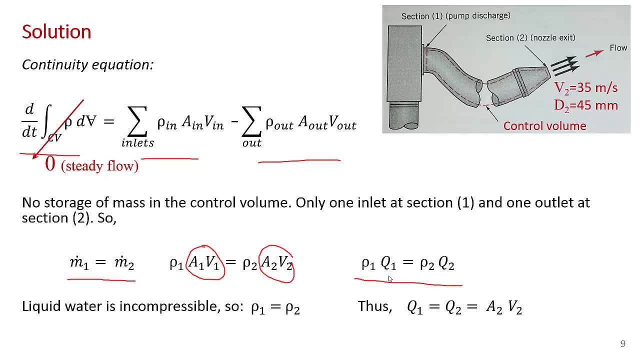 in this form where rho one times the volume flow rate at one equals rho two times the volume flow rate at two. Now, in this case we're talking about liquid water. Liquid water is incompressible. it density doesn't change with pressure. so rho one equals rho two and we can cancel that term. 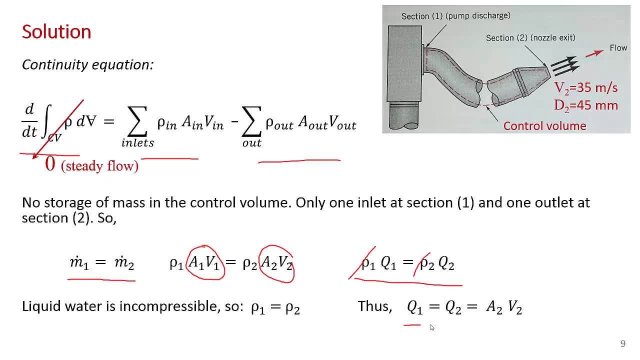 with that term. And so we just end up with the volume flow rate at one flow rate in the hose is a constant q1 equals q2 and in fact at any cross section we have the same flow rate. and since we have the area and velocity at,